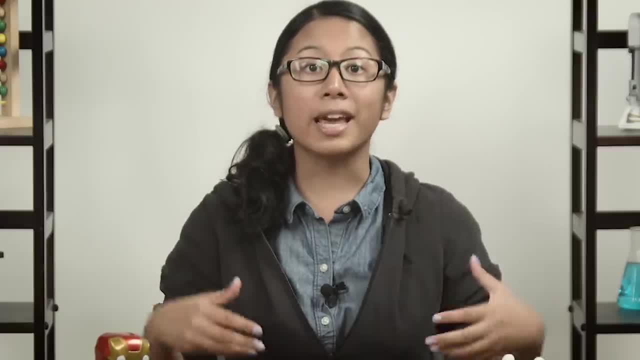 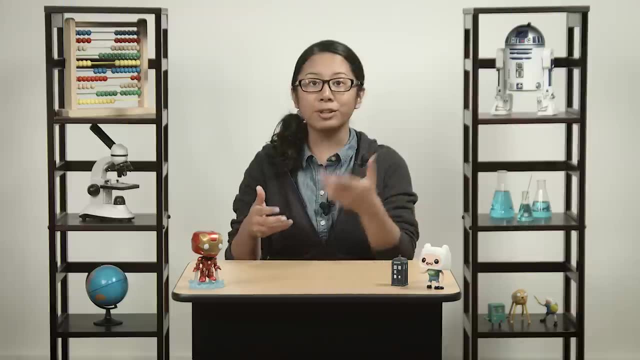 live And I need a place to film Crash Course videos. You could say this is my habitat. Animals need these things too: Food, water, shelter and space to live For animals. their food comes from their neighbors, the other living things in their habitat. You know that plants and animals all fall. 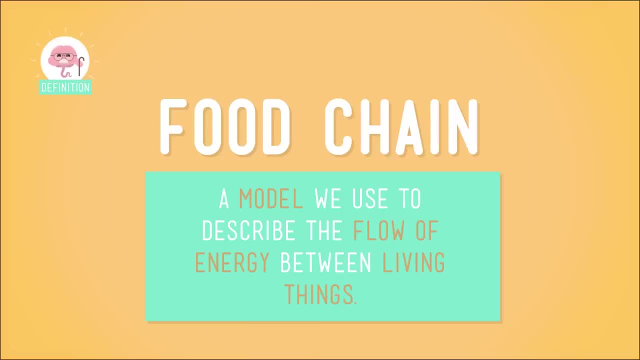 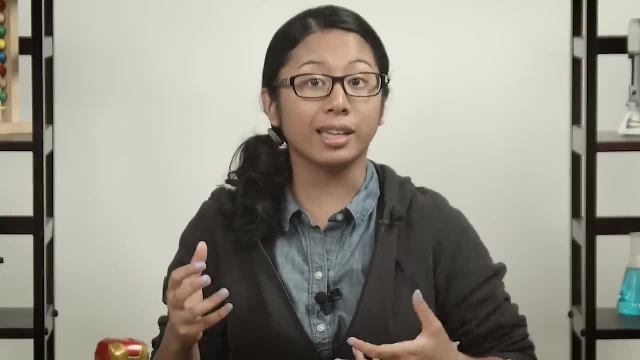 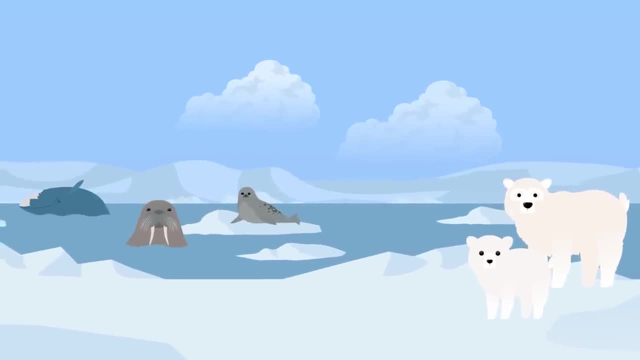 The world is made up of lots and lots of food chains, and those chains can get kind of messy. I mean, look at our polar bear. Sure, his favorite food is seal, but in a pinch he'll eat walrus, dead whales, bird's eggs and, if he has absolutely no other choice, plants. The polar bear is at the top of multiple food chains, and that's not unusual. Most animals don't just eat one thing, and neither do I. I'm at the top of the pancake food chain and the carrot food chain. It just so happens I prefer pancakes, So you can see how. 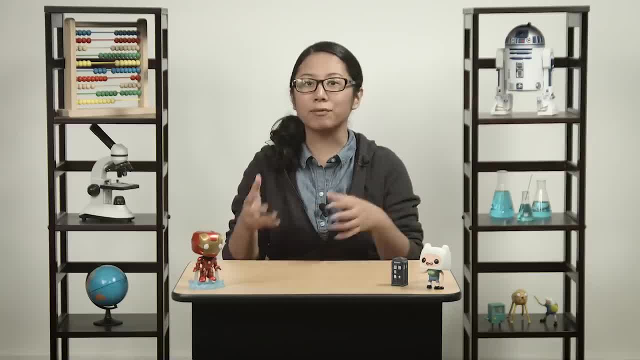 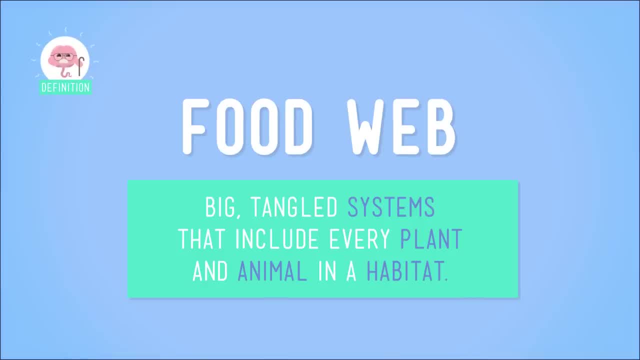 food chains are actually all tangled around with each other, with many different ones overlapping, kind of like a web, So we call this a food web. Food webs are big tangled systems that include every plant and animal in a habitat And, as you might guess, all. 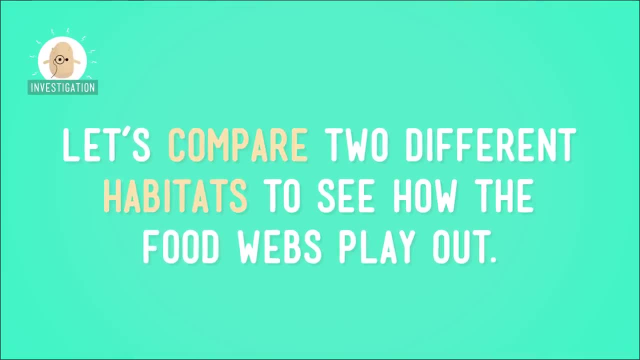 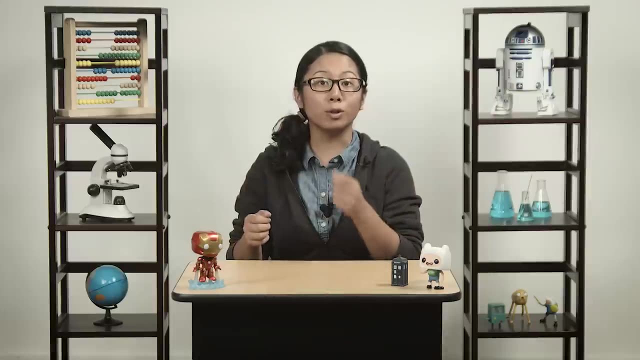 food webs are different. Let's compare two different habitats to see how the food webs play out. First we'll go back to our old stomping ground, the forest. Let's begin with- you know this, people- the plants, Trees. 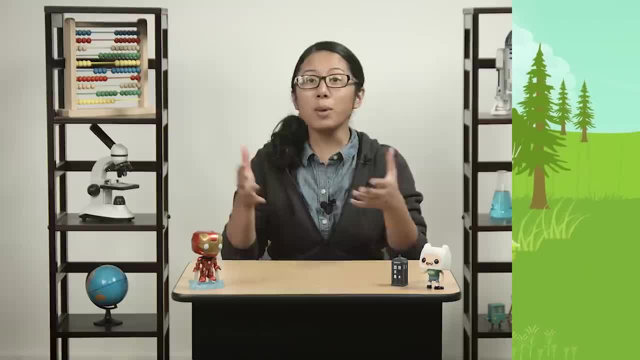 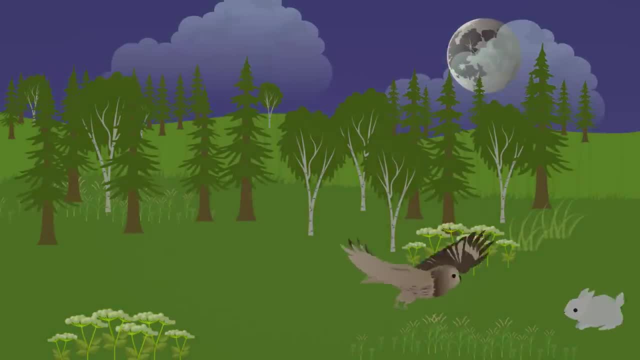 grass and other plants that change energy from the sun into sugar. But then you have some animals that eat other animals. This is where things get a little more complicated. Today an owl makes a mouse his lunch, but tomorrow it may be a rabbit. Today a snake snacks on a squirrel, but a few days later our owl friend. 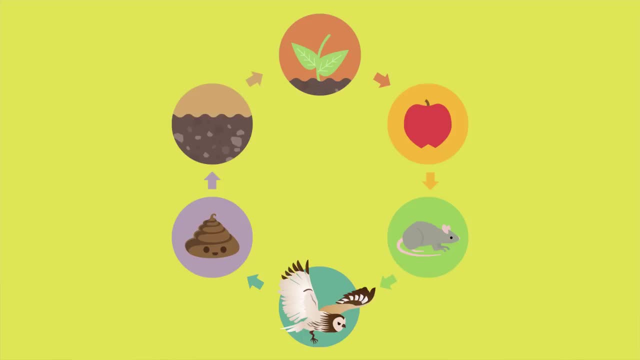 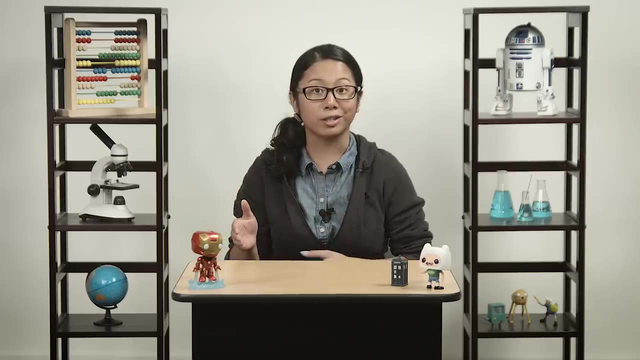 might make a meal of another meat eater like the snake. Finally, the decomposers- insects, fungi and bacteria- are breaking down whatever's left over, from uneaten rotten fruit to leftover animal carcasses. As they break down matter, they provide more nutrients for the plants. 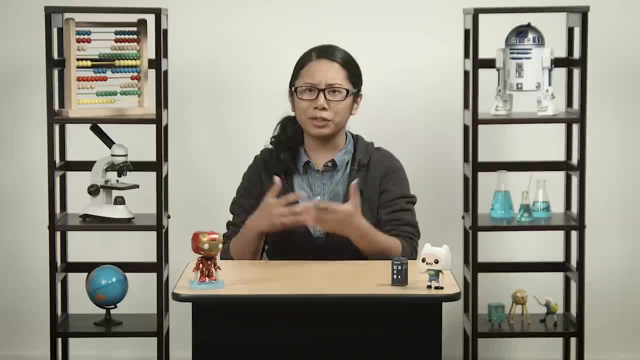 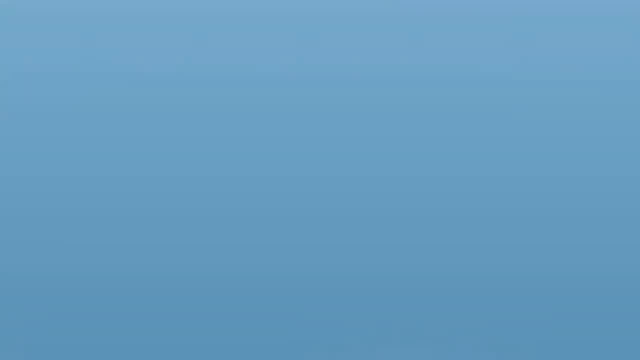 Kind of a different story up in the Arctic. I mean, look at all that ice. I know what you're thinking. Where are the plants? How do we have a food web without plants? Zoom in on the seawater. Zoom way in Further, Further Stop. Can you see those tiny plants? They're called phytoplankton and, just like plants on land, they convert energy from the sun. Really small creatures called zooplankton eat the phytoplankton and all kinds of small fish dine on the zooplankton. Larger fish eat the smaller fish. There are big marine.